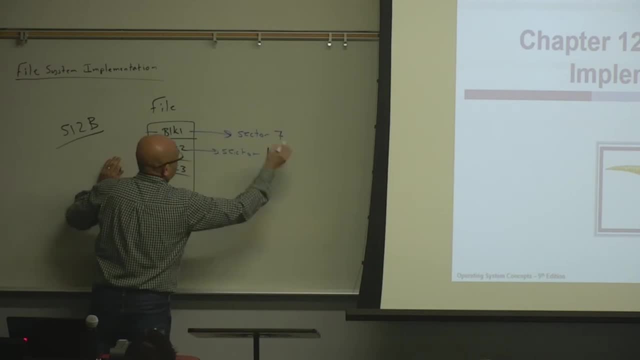 And this could get mapped into sector 101.. So, just like memory management And Logically, the file here is a contiguous sequence of blocks, But physically, on the disk, these blocks can be scattered all over the disk. They don't have to be contiguous. 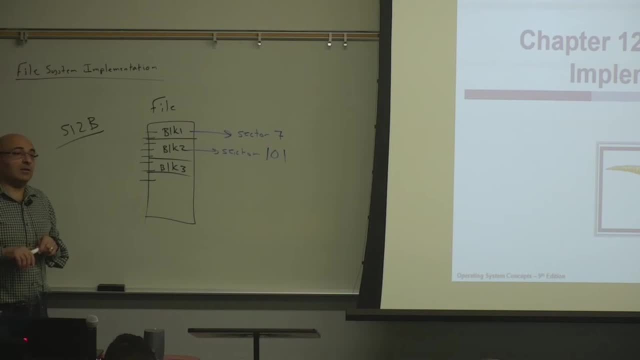 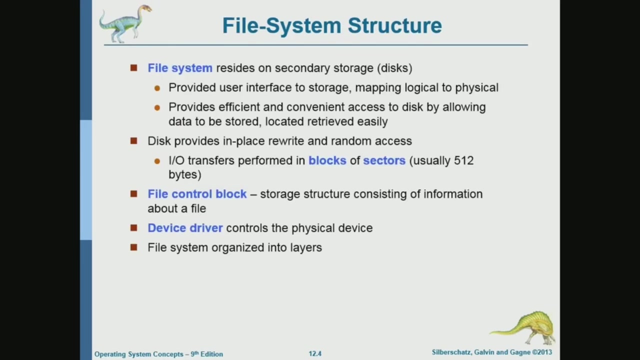 And they don't have to be in order, Right, So mapping blocks into sectors is just like mapping pages into frames. in memory management, Okay, And in file system implementation, one of the important data structures is the file control block. We'll see more details about this later in the day. 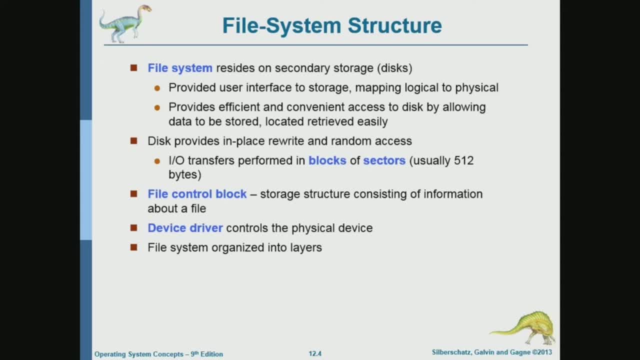 So the file control block is just a block data structure that the operating system keeps, or the file system in particular keeps, to store information about each file. Okay, And the device driver is another important component. The device driver is that part of the operating system. 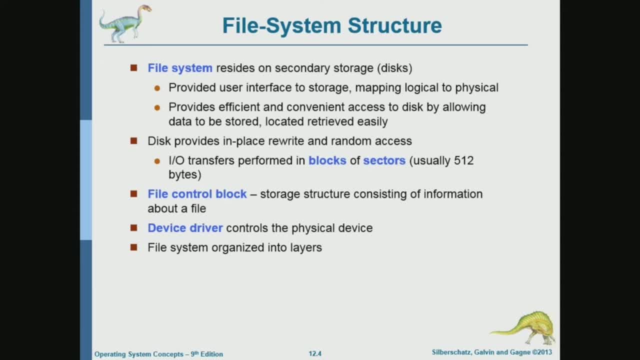 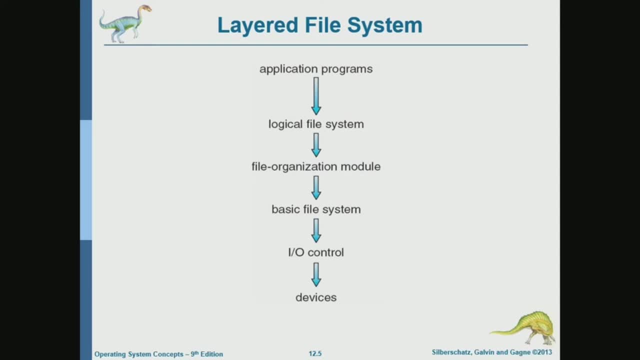 that talks to the hardware. Okay, That controls the hardware. So a file system is typically organized in layers. Of course, every file system is different, But this is sort of a generic organization of a typical file system, or it's something that is common. 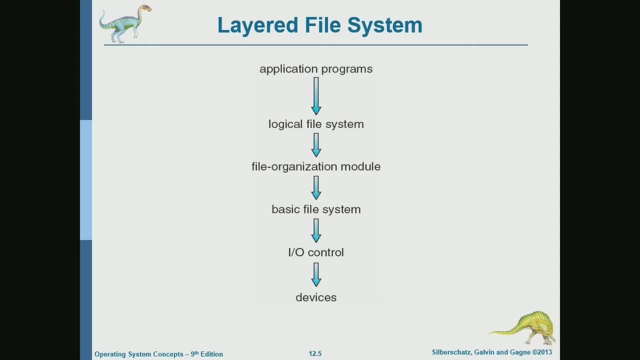 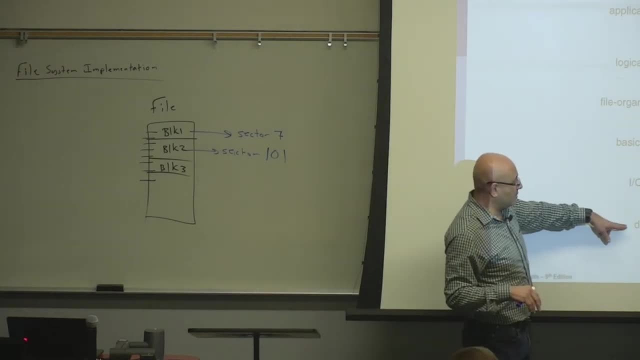 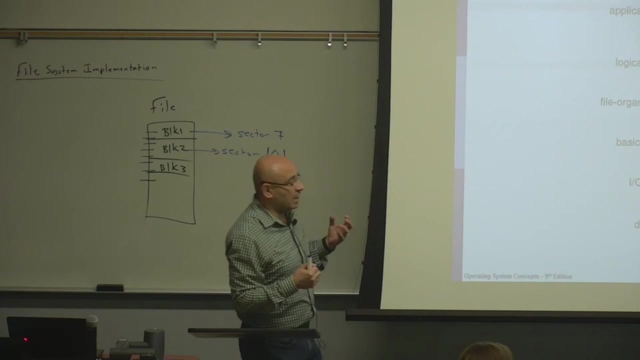 to most file systems. They are organized in layers, So the bottom layer is the low-level layer that talks to the hardware, which is the well. this is the devices, the actual device, the hardware. By the way, when we say devices or device in the context, 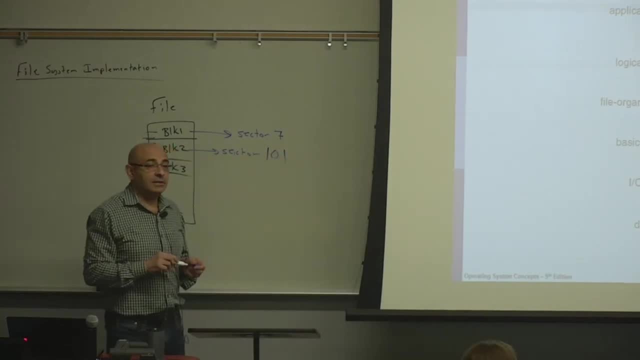 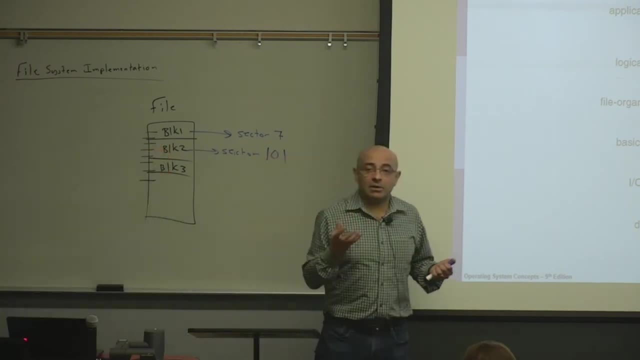 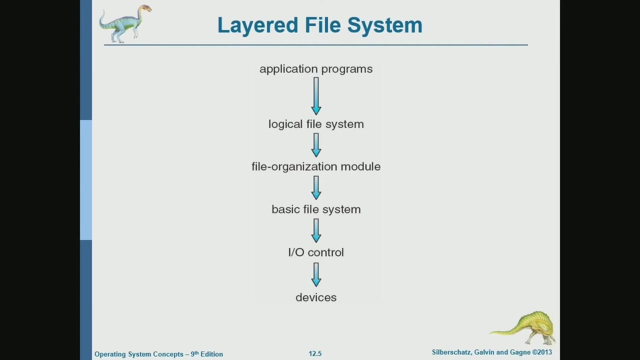 of file systems. what kind of device are we referring to? What's the device that we're talking about in file systems? The device that we're talking about here is the disk. So the IO control layer is the layer that controls the hardware. 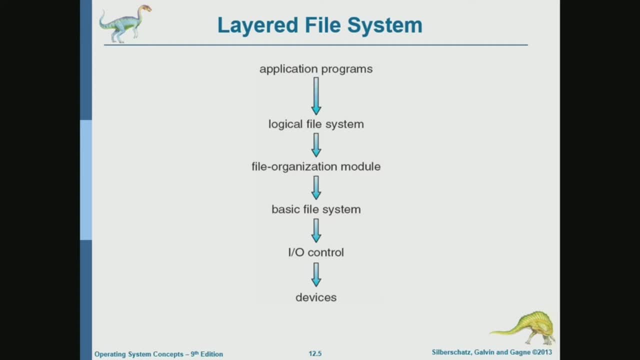 And there is, on top of that, the basic file system, on top of that, the file organization module, on top of that, the logical file system, and on top of that we have the application. Now, the next slide. you will see what each one of these means. 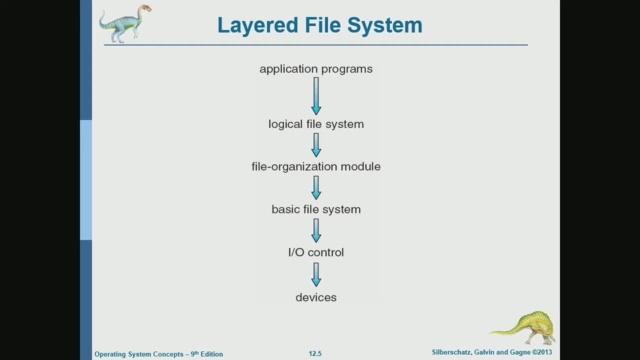 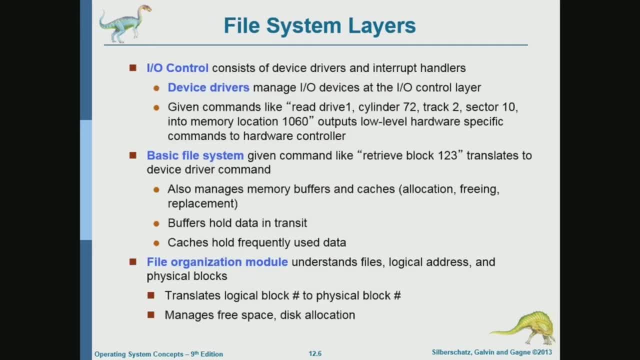 So the lowest level is the IO control, which is the device drivers. This is the lowest level layer that talks to the hardware, And this layer receives commands like read from drive 1 with a cylinder number, track number and sector. So this is the address on this. 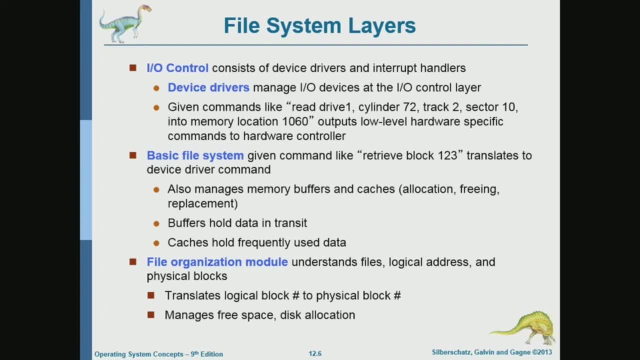 The address on this. you first specify the drive number, because you may have multiple drives, And within each drive you have a cylinder number, track number and sector number. okay, Now this layer will translate these into low-level commands that are machine-specific or that are device-specific. 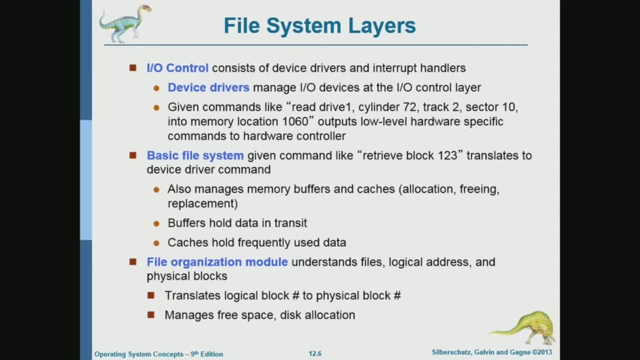 not machine-specific. They are device-specific commands that will access that particular sector. okay, On top of that there's the basic file system layer that receives requests for physical blocks, like you know, block number 123. So block 123 in this layer will get translated. 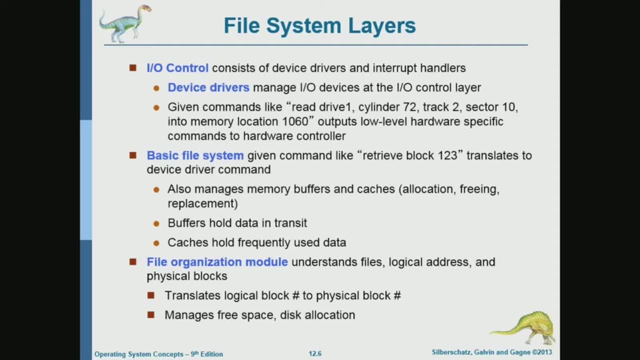 into the system-specific command: Drive number, cylinder number, track number and section sector number- and this command will be sent to the IO control layer And this layer will also have the buffering, the buffers that will buffer data, that will get transferred. 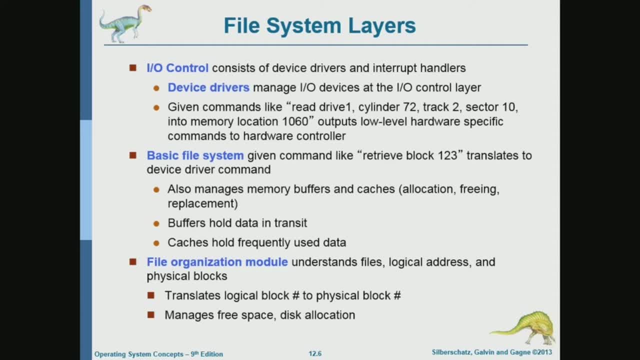 between disk and memory. Now on top of that there is the file organization layer. Now you may have noticed that in layers in the IO control and the basic file system layers we don't have the notion of a file. So these layers don't know about files. 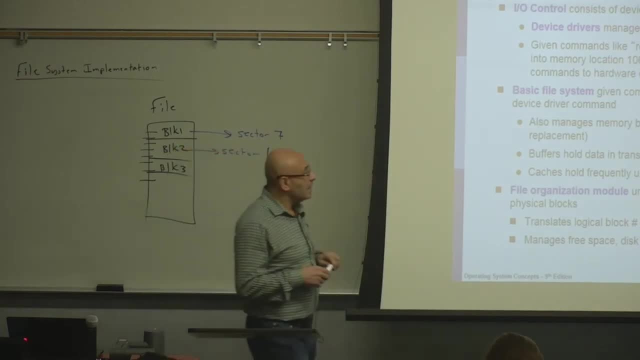 They know about blocks. okay, Now this layer knows about files. So this layer is going to translate logical blocks into physical blocks. So now, what do we mean by a logical block here? A logical block is, like you know, block number 5 in file XYZ. 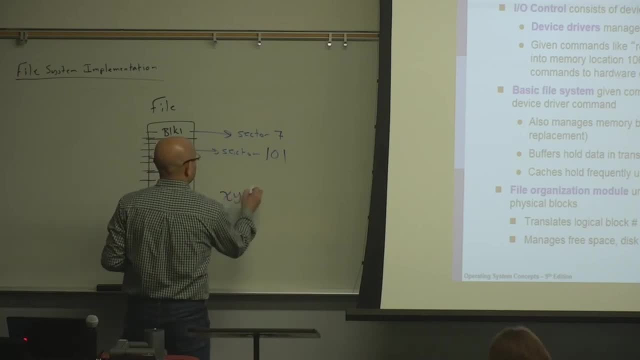 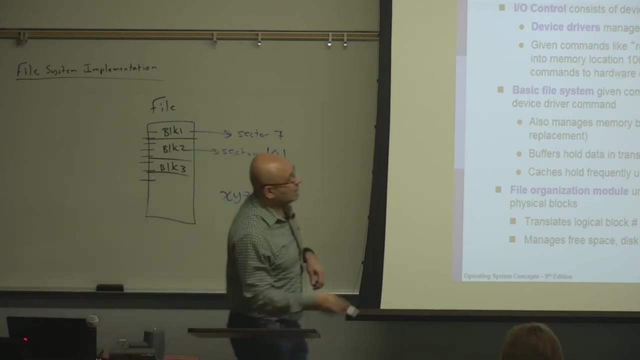 So block 5 in file XYZ will be, for example, block you know, 123.. So block 5 in file XYZ is will get mapped to some physical block number And the command will be sent to the lower layer. okay. 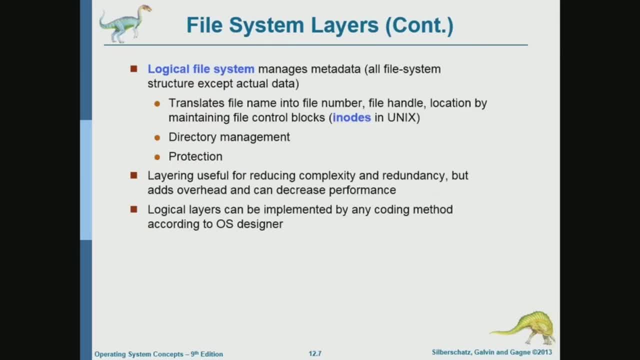 Now the layer on top of this, the logical file system layer. so this is basically the directory level layer. So the previous layer was the file level. here, On top of the file level, you have the directory level, because the directory consists of multiple files. okay, 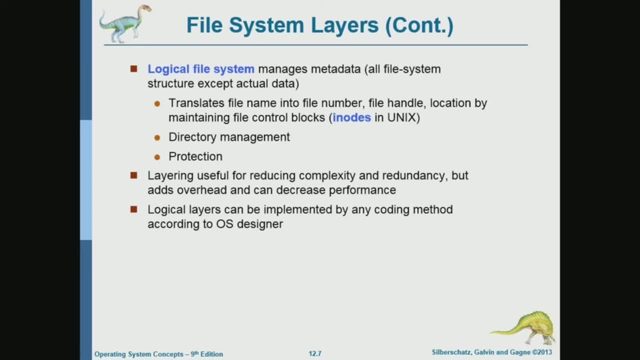 So it's, you know, this layer, you know, manages directories. It will have the directory structure And in the directory structure, as we will see, there is a, there is an entry for each file And there is a file control block for each file. 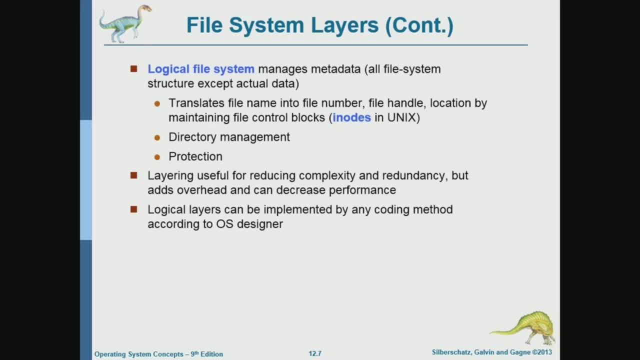 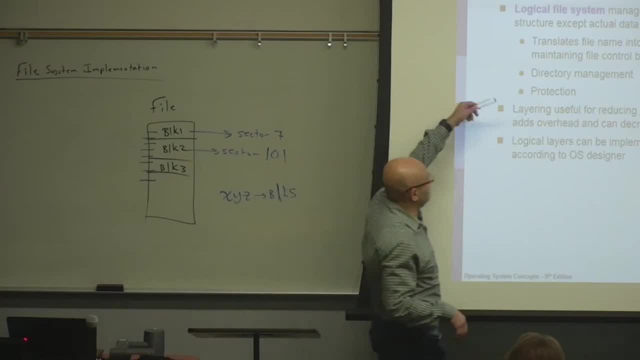 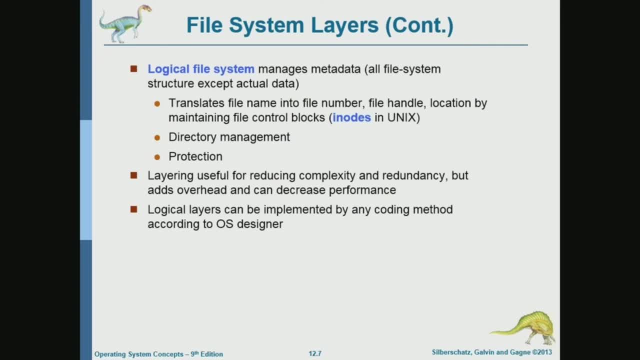 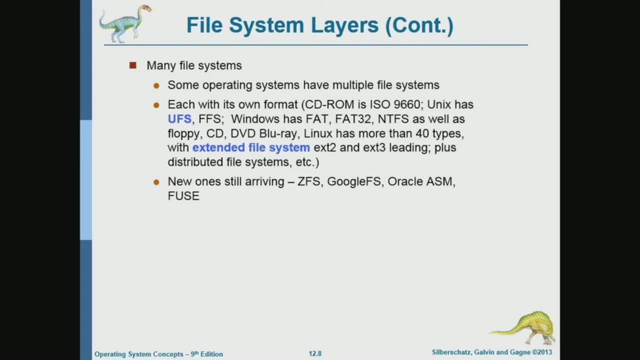 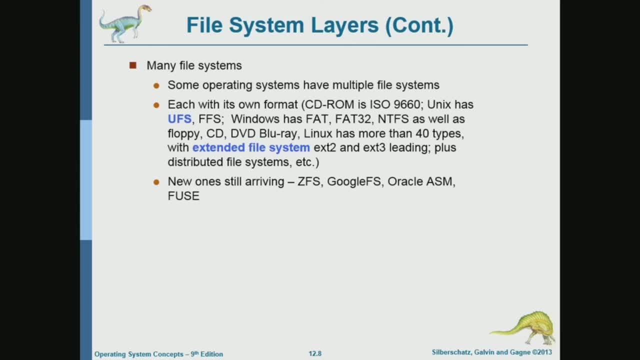 And it shows that one operating system may have multiple file systems, like Windows, for example, has FAT, the FAT file system and the NTFS. Okay, Yes, So you respect. yeah, And people are still coming up with new file systems. 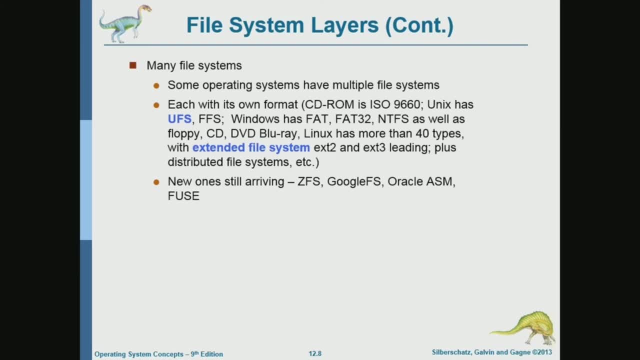 so new file systems are getting, you know are still arriving, like the Google file system. So file systems, we have a lot more file systems than operating systems. you know Operating. we don't get new operating systems very often You know even a new operating system. 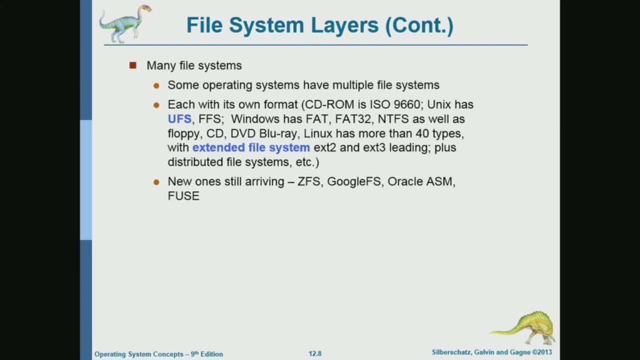 like. Android is not a totally new operating system. It's based on Linux, So it's not a brand new operating system. It's a mobile version of Linux. That's what Android is, So it's file systems. we only have a limited number of. 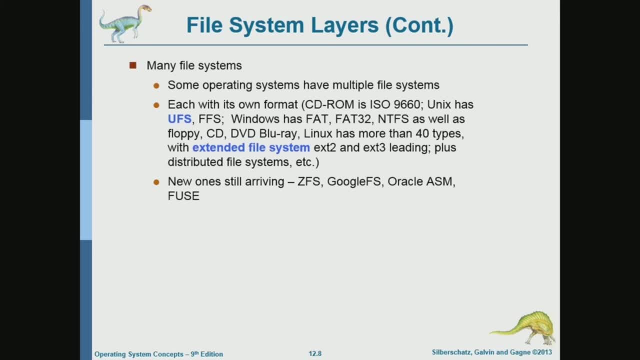 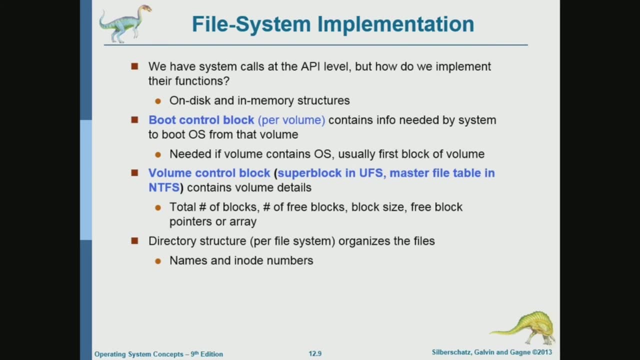 sorry, a limited number of operating systems, but we have a lot more file systems And you know the file system is just a, a subsystem of the operating system. Now, the implementation of a file system in the file system has data structures on disk. 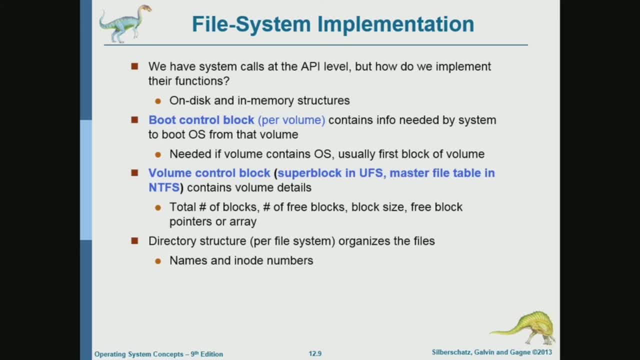 and data structures in memory, So on disk. there is there are data structures that are kept on disk and data structures that are kept in memory, So on disk. there is the boot control block, for example, per volume, So this has information about how to boot an operating system. 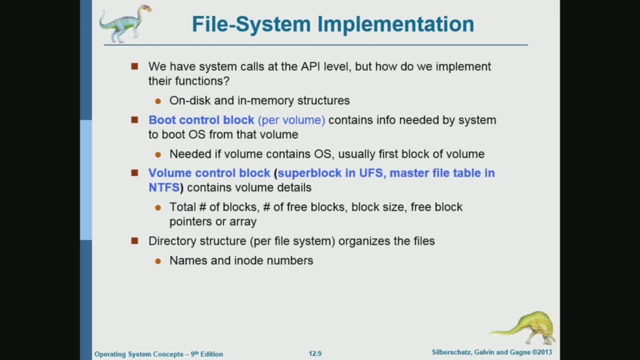 if that volume has an operating system, if it's a bootable volume- And we know that we can have a, you know, a volume can be bootable or unbootable depending on whether it has an operating system or not. So if there is no operating system, 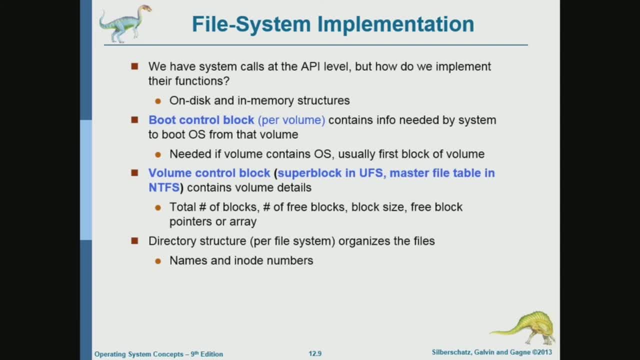 this block is going to be empty. There is the volume control block. For each volume, there is a block that has information about the number of blocks, the number of free blocks, the block size. It also has the directory structure. It also has the directory structure. 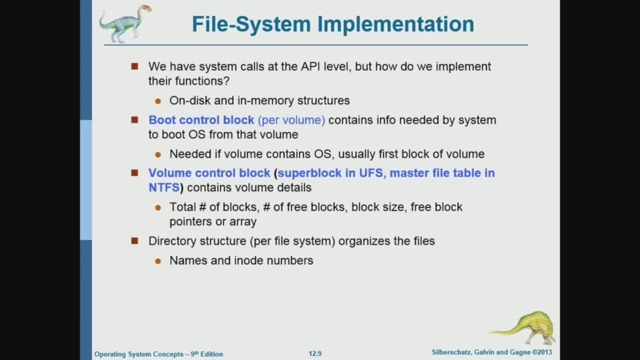 Sorry, the directory structure is another thing. So volume control, blocks and there is the directory structure, which is one directory structure for a whole file system. And what the directory structure has is the directory structure has the file names, or you know, the directories and the file names within each directory. 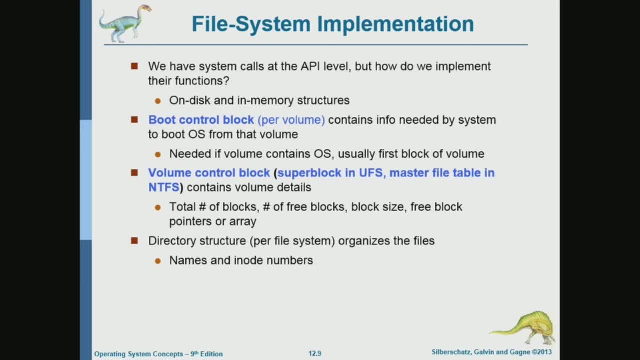 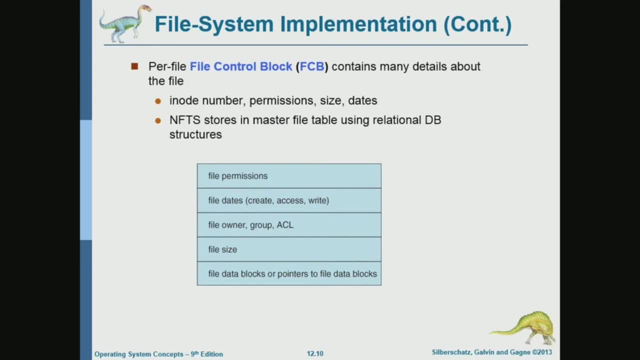 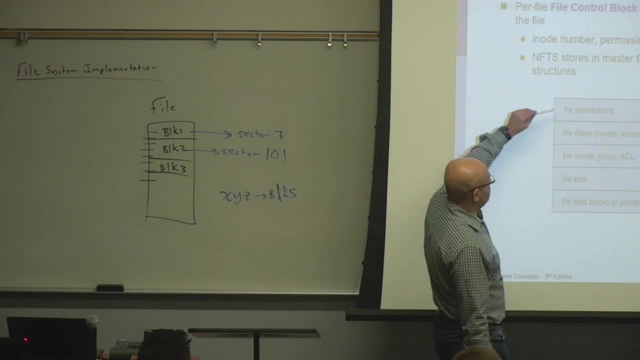 And for each file there is a file control block. What's in the file control block? The file control block the information that the file system tracks for each file, including the permissions, the dates when the file was created, when was the last modification. 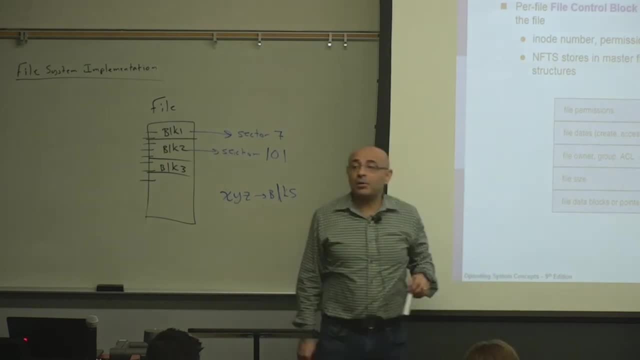 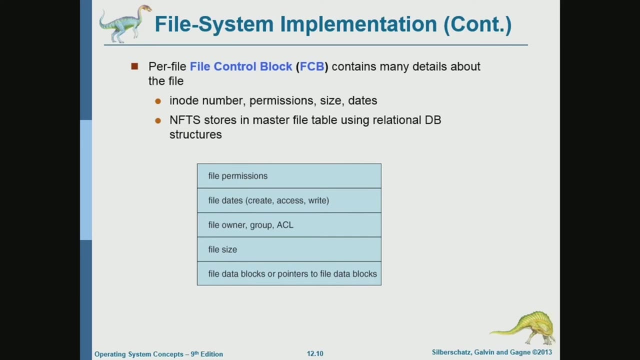 the owner of the file, the size of the file and pointers to the actual data blocks. The file control block doesn't have the actual data, It's just a header. It has the information about the file and it has pointers to the actual data blocks that constitute that file. 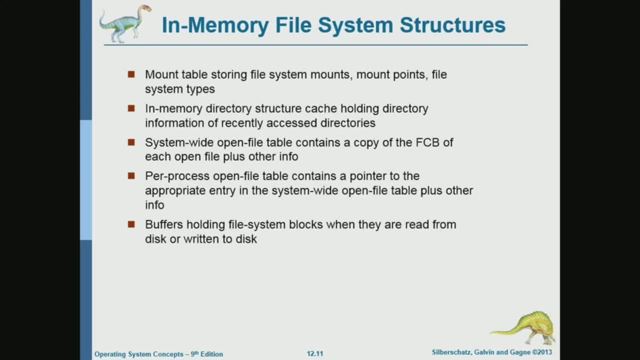 Now, what does the file system have in memory? The file system has in memory the mount table. so the mount table has the will have the different drives that are mounted or the different volumes that are mounted to that file system. It will have in memory a cache of the directories. 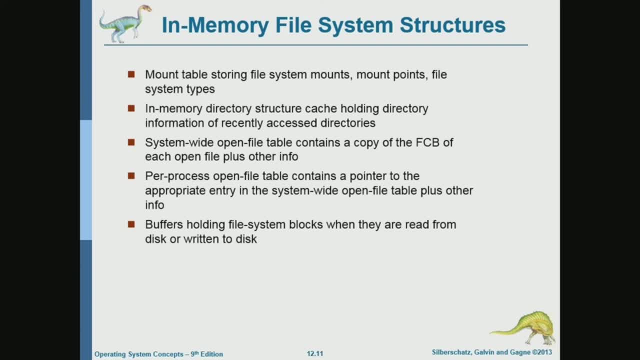 that have been accessed recently. So you can have a whole directory structure And it doesn't make sense that you load information about all directories in memory, Because typically you know if you have a one terabyte drive it has lots of directories and lots of files. 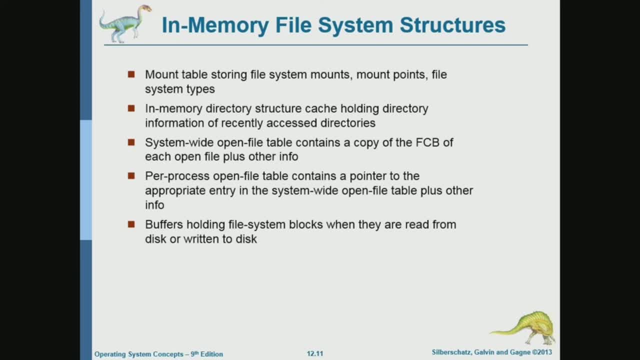 And it doesn't make sense to load information about all of them in memory. What you need in memory is the is loading information about the directories that have been accessed recently. So it's sometimes it's caching Caching, So you need to have frequently accessed directories in memory. 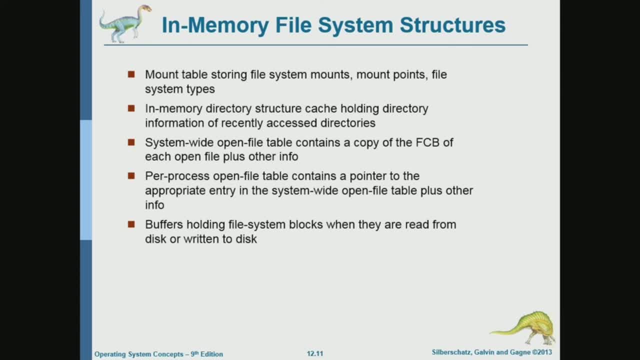 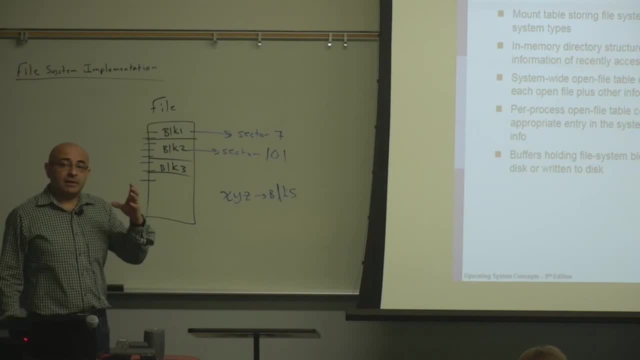 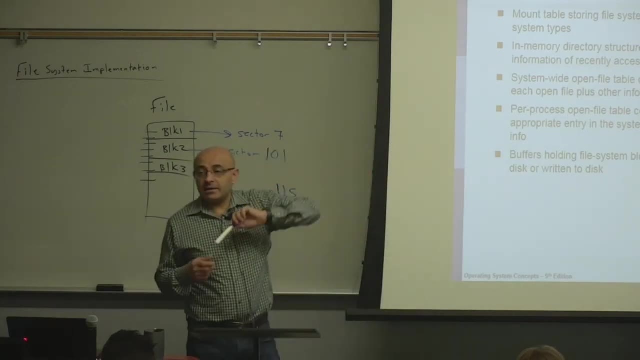 There is a system wide open file table and there is a process wide or pair process open file table. What's the open file table? It's a table that has information about the open files. The system wide table has a copy of the file control block. 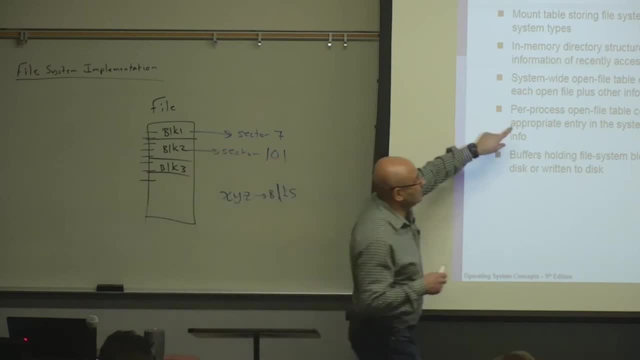 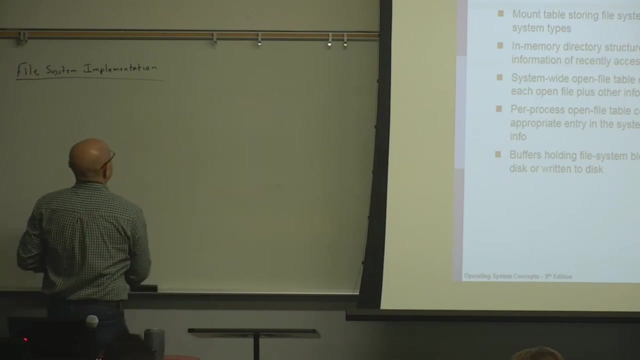 for every open file, The pair process Open file table will have a pointer to the corresponding system wide. So why is that? Because a file may be opened by multiple processes. So if you have a certain file that is open by multiple processes, so this is the system wide table. 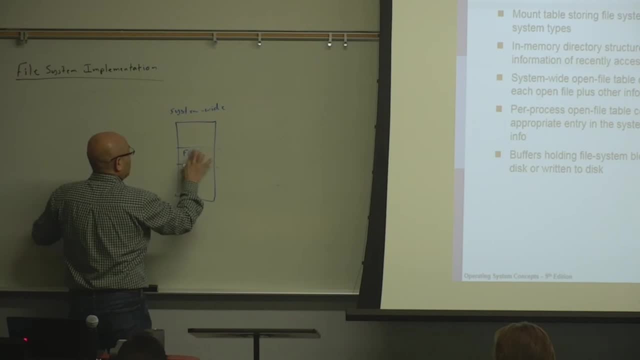 So the file control block- file control block for, say, file X- will be in the system wide table. Now if you have two processes- process one and process two- that have this file open, each one of them will have an entry in its pair process table and they will just point. 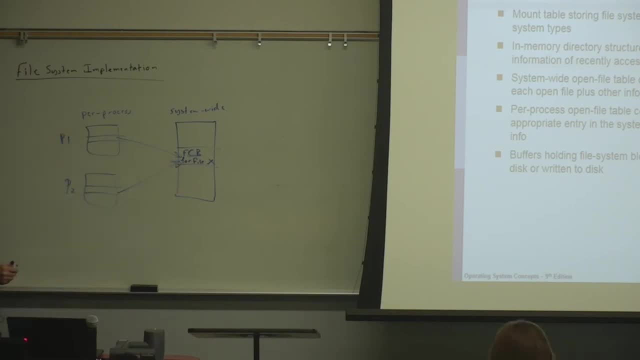 both point to the file control block for that file And the system wide open file table. So in other words, you don't have to have a copy of the file control block for each process. So there, because there could be multiple processes opening. 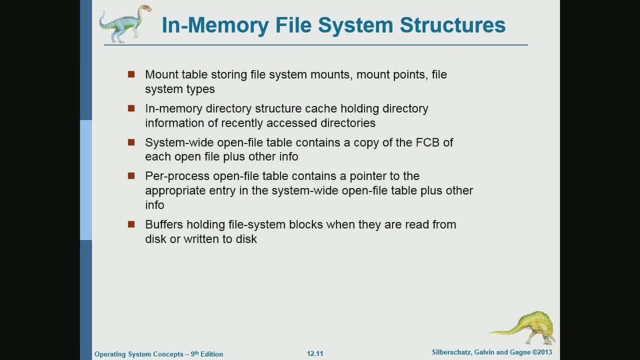 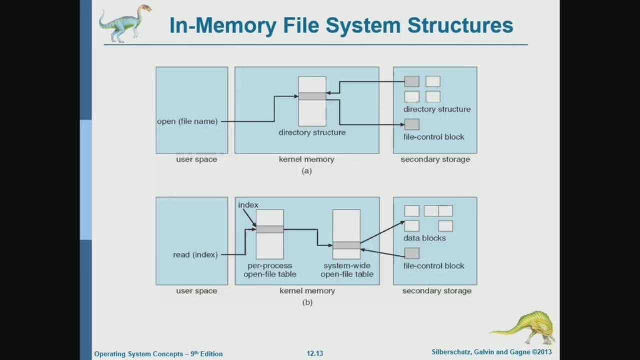 that file. Okay, And there are, you know, buffers that the system uses to buffer the transfer of data between disk and memory. So let's look at, Let's look at these pictures that will show what happens when a file is opened, when we open a file. 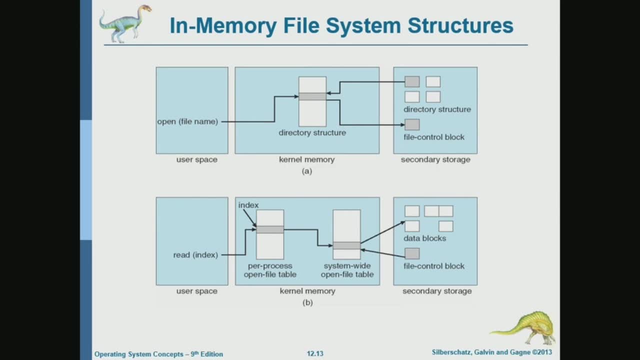 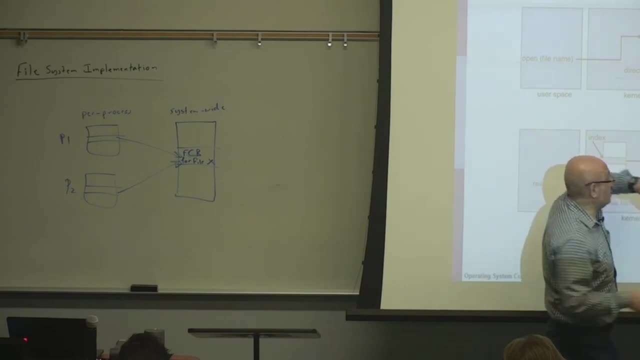 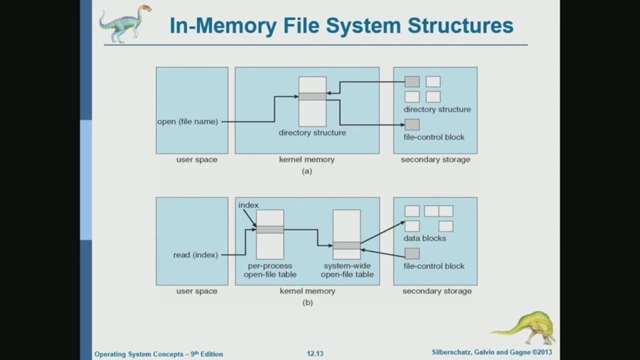 So when we open a file, this is the directory structure in memory. so this is user space, this is memory. of course, kernel memory, So these are kernel data structures And this is the disk. Now, if an application you know makes a system call, 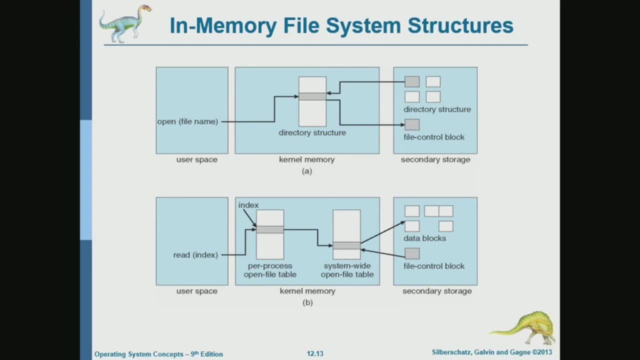 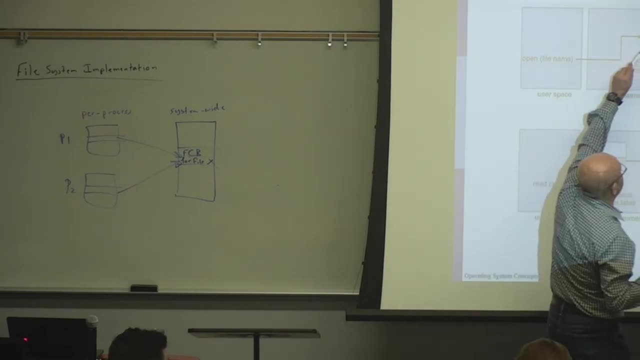 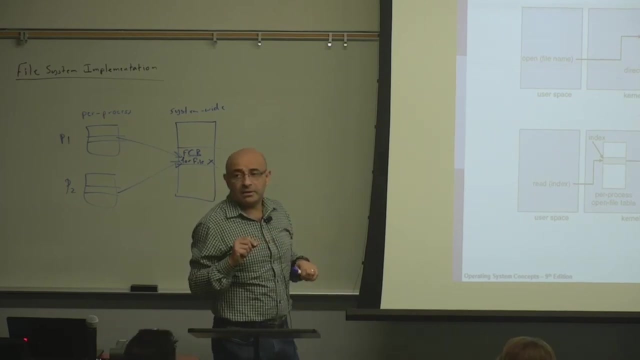 to open a file you know. assuming that you know the directory entry for that file is in the directory structure, it will get used, Of course. if it's not there, it will get loaded right. So if that directory is cached in memory it will get accessed. 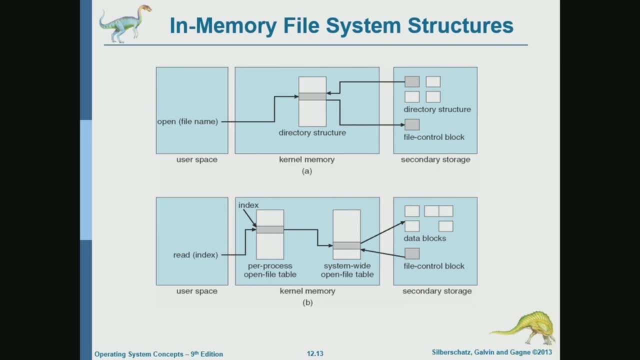 If it's not cached in memory, the system is going to load it from disk. So it's going to load that information for that directory into the directory structure, if it's not already there, And then it will look up. you know that file name within that directory. 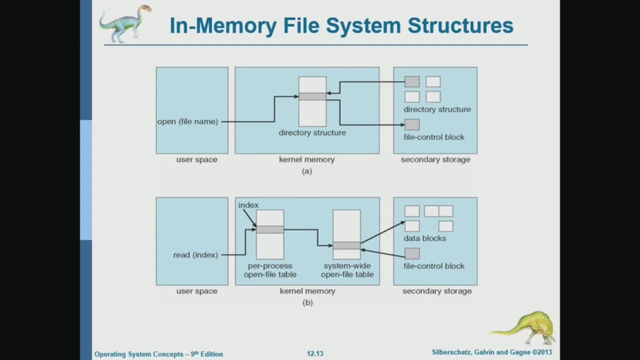 So the directory will recognize file names and each file has a corresponding number. So, like if the directory has 100 files, these files will have numbers from 1 to 100, but you are sending request for a name, So it will map the name into a number. 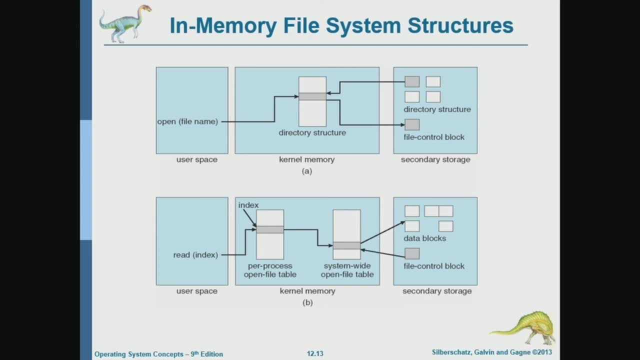 And it will go to. you know, if it's file number 17 in that directory, it will go to the file control block for file 17,. okay, Now when you read from a file. now when you read from a file. 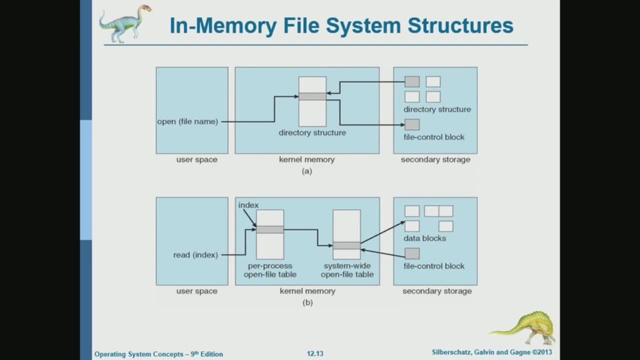 you will need to access the actual data blocks. So now, when this file gets open, there will be the file control block, for that file will get cached into the system-wide open file table. So the file control block will be in the system-wide open file table. 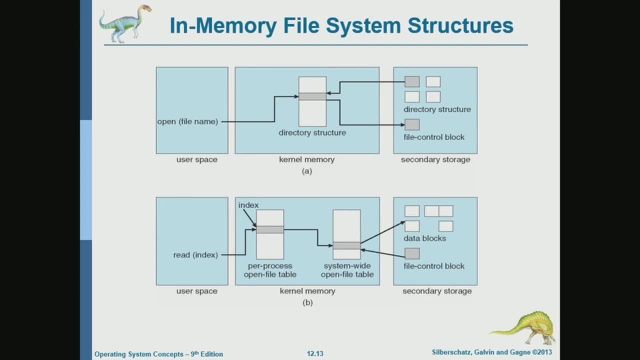 And the per process open file table will have a pointer to that. okay, And that file control block for that file will have the pointers to the actual data blocks, okay. So that's. this just shows us how you know things. you know what the file system has on disk. 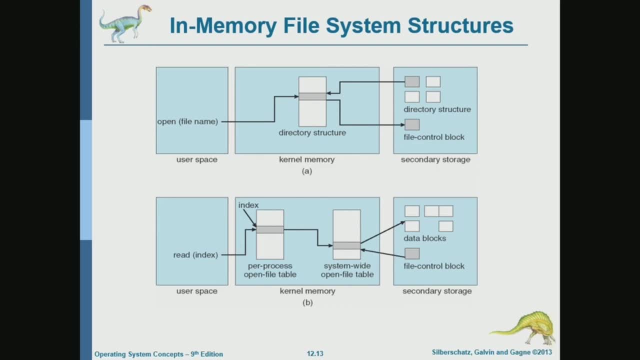 and what it has in memory. So basically it caches the things that are accessed in memory. Anything that gets accessed gets cached into memory, But it definitely- you know- doesn't load everything on disk into memory. There is no reason and there is no room for it.